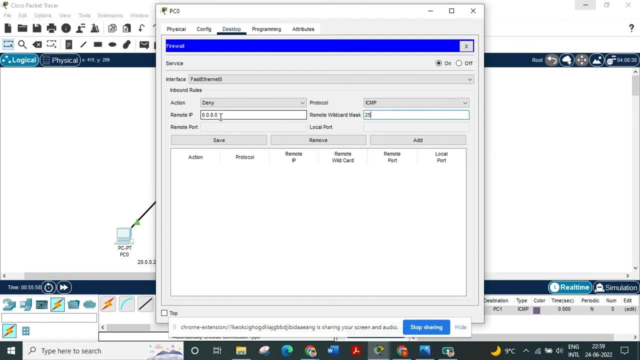 be 255.255.. Same number, same number. Then we press add: Okay, so we are going to not allow the ping service between these two pieces. But what if I want to allow PC0 to access PC1's IP address but not interact with each other through ping service? So we have not allowed. 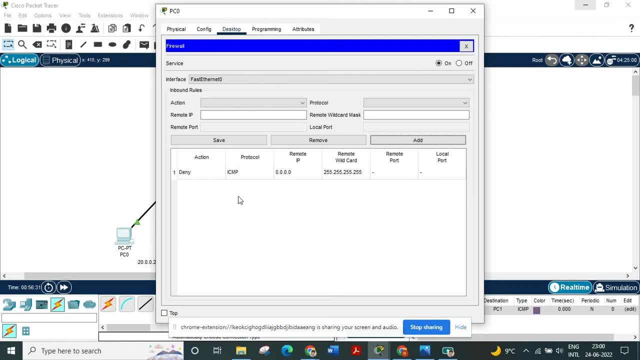 the ping service. but we are going to allow the IP addresses of both the pieces to view each other's IP address. To do that, press allow. And we will also change the IP address of PC, say PC1,했던 weiß. 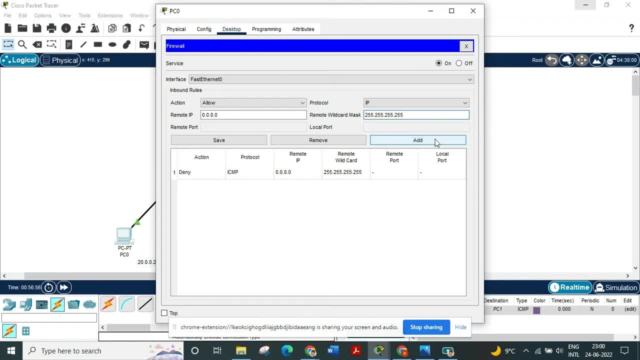 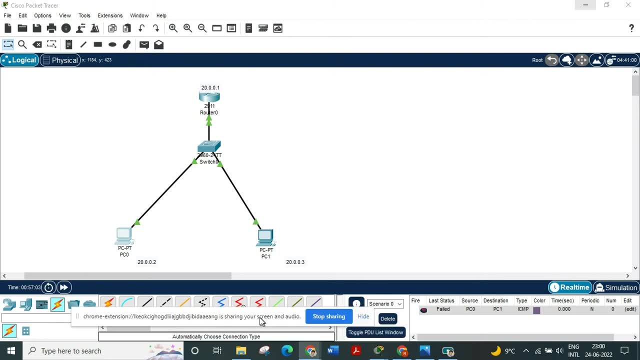 up to PC0. It's whatever your account is. So it's reduces ingress 2ologne again, If we want to go ahead and check just now. so thisguysolynet is government address to架 swallowth terribly. Let's type this: And it says that the pin status of PC0: 0.0.0.0.0 to PC 1.0.0.0.0, to PC1.0.0.0, to PC1 clock è. 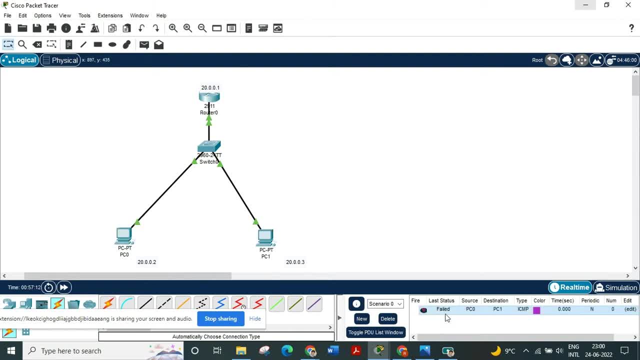 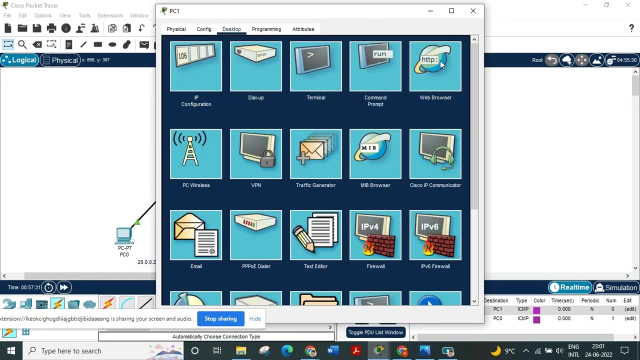 failed. why? because you have set up inbound role rules in the firewall section of pc0. that's why we're not able to use the icmp services. but let's check if i'm able to access the ip address of pc0 from pc1's web browser, and the ip address of pc0 is: 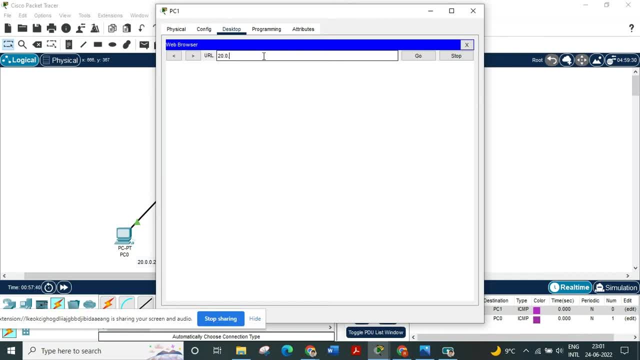 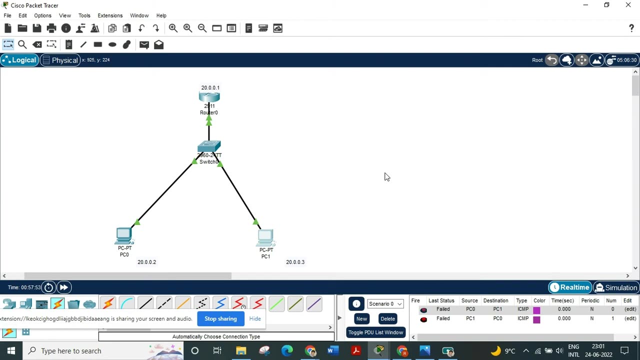 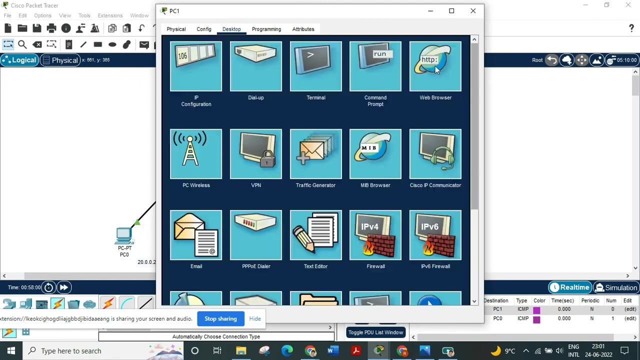 20.0.0.2. let's go, it's our reset connection, okay. so yes, we are successfully able to access the ip address of either of the pcs, but just not able to ping each other for safety reasons. we can double check. we can go to command prompt and.